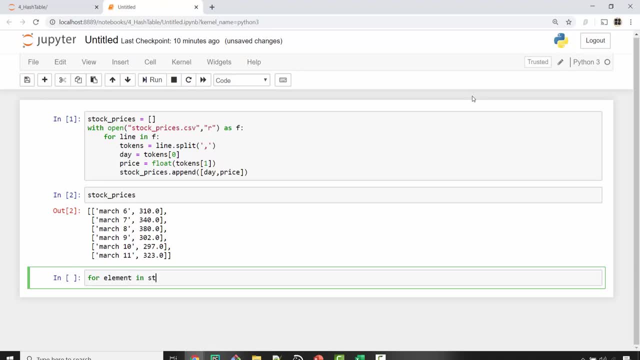 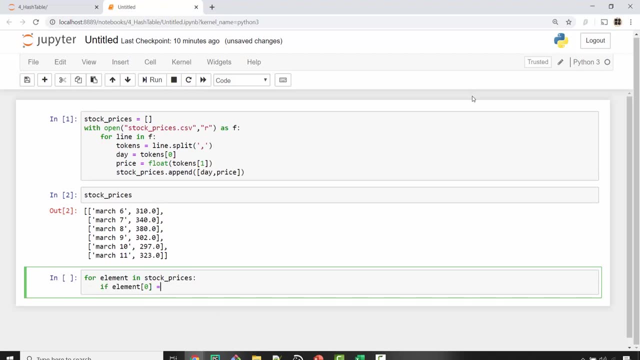 for loop saying for element in stock prices. if element zero is equal to march 9, then you have found your element. so print element one. so this program tells you that on march 9.. the price was 302. while using a list works here, but it is not very efficient because imagine: 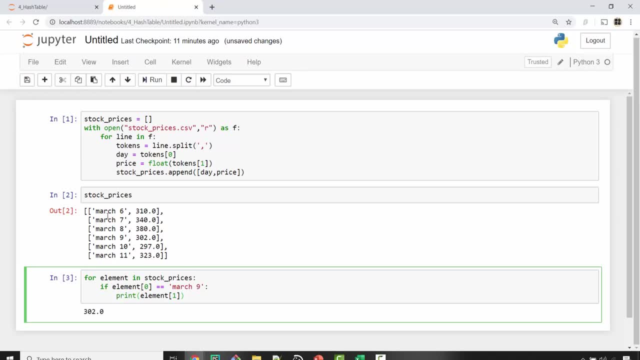 if your file size is, let's say, million records and the date that you are looking at is towards the end, then you have to run those many iterations. so the complexity of this program is order of n. to find a price based on a day, it is order of n. complexity in python. there is dictionary which 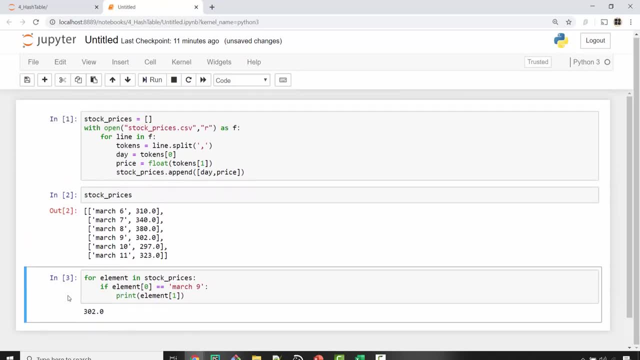 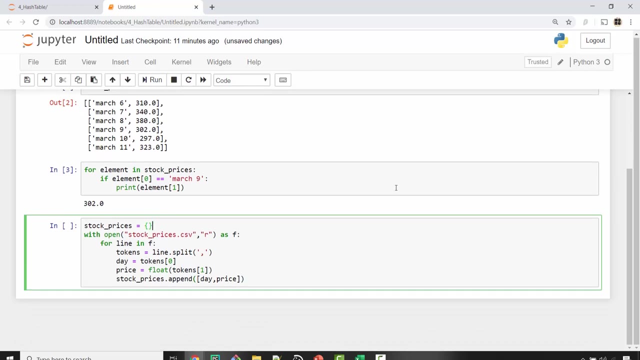 can do the same thing in order of one, which is a constant time operation, and let me show you how you can do that. so here i'm gonna copy the same code, and one change i'm making is replacing list with a dictionary. so my stock price is: 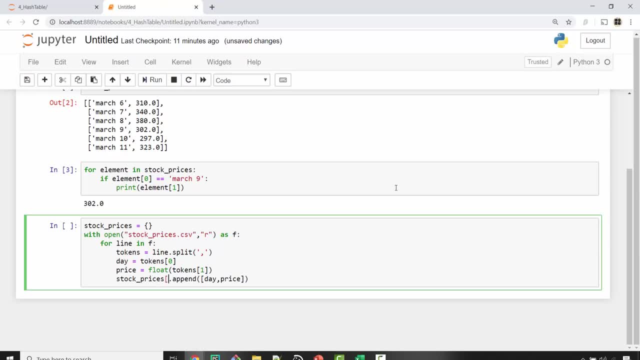 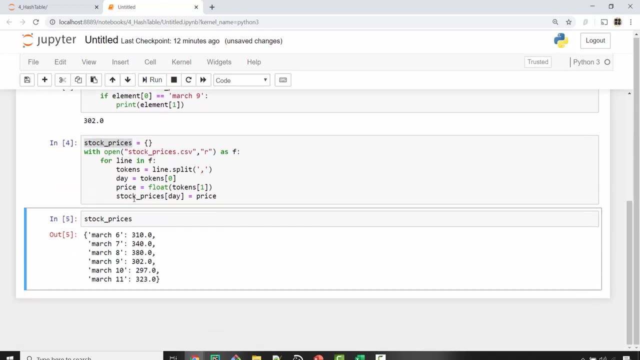 is a dictionary now, and if it is a dictionary, you know you can add a key by using this index operator and you can just say: that thing is equal to price. okay, and when you print the dictionary it looks something like this: where each of the days are key and then you have value as a price. 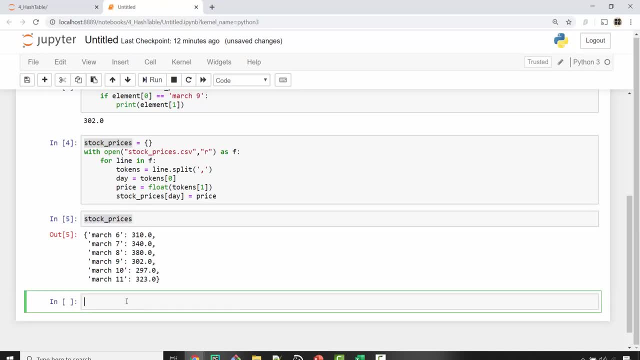 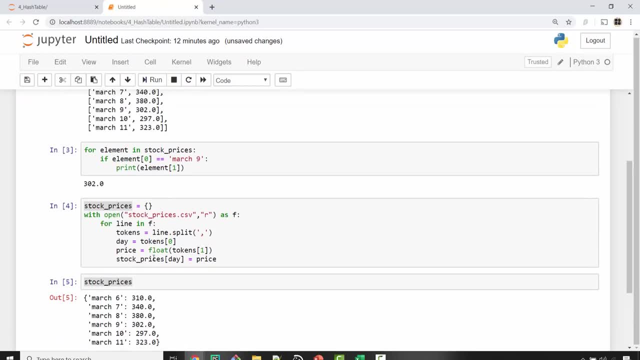 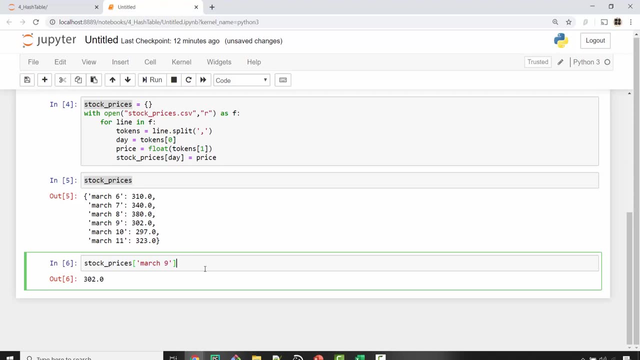 here, and you can see that in this particular case, using dictionary makes more sense because this operation is order of one. now we are going to look into internal implementation of a dictionary. so dictionary implements hash table. so hash table is the underlying data structure, and we will see how. 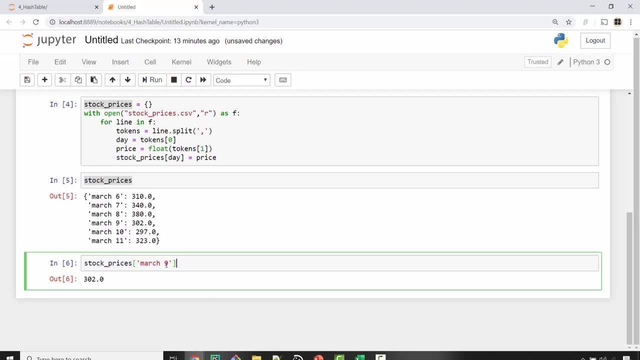 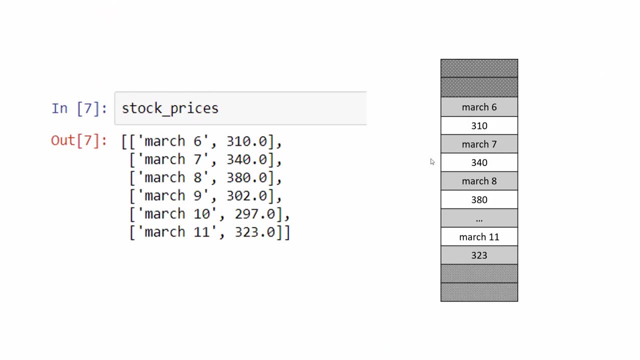 you can get order of one and you can get order of one and you can get order of one and you can get close to n equation. so this type: if you get the first and last part, you get codeled. end of the the object. so and or 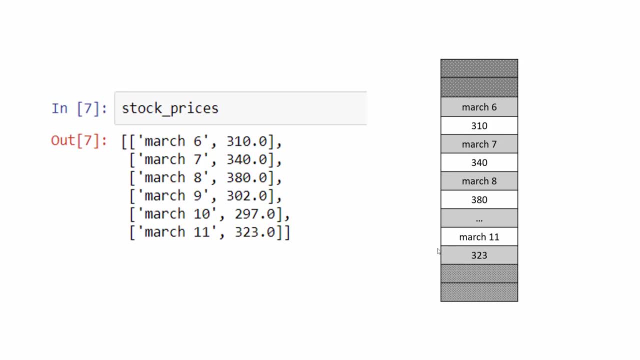 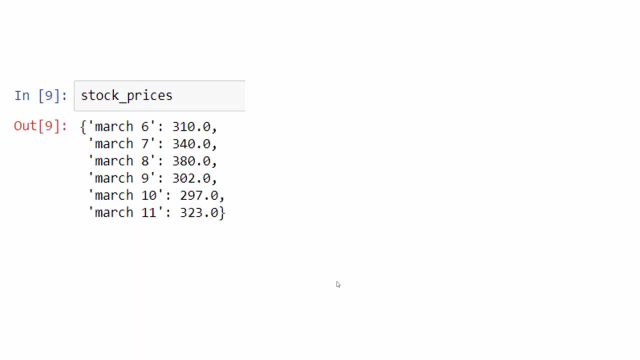 and ah, let's say it will allocate a list of some operating quit and size, let's say a size of 10, and then it takes March 6 first. somehow it will map March 6 to a specific element in the list and to get the index of the element. 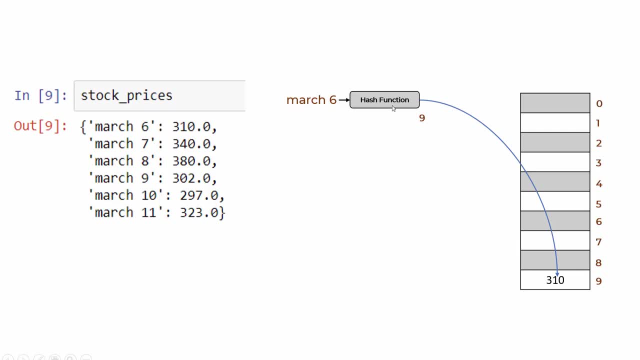 in that particular list. you use hash function and we will see what this has function is later on. but all the hash function is doing is converting your string key into an index into an array. similarly, you can apply hash function for all other keys, find out an index into an array and store those elements. 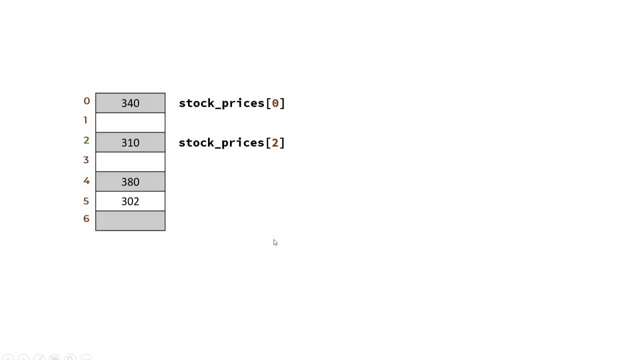 at that index. so it is that simple, okay. so if you think about it, if you're an array, usually you use integer index, correct? so let's say: this is my array, my integer index is 0, 2 and so on. in hash map all you have is a string index. so 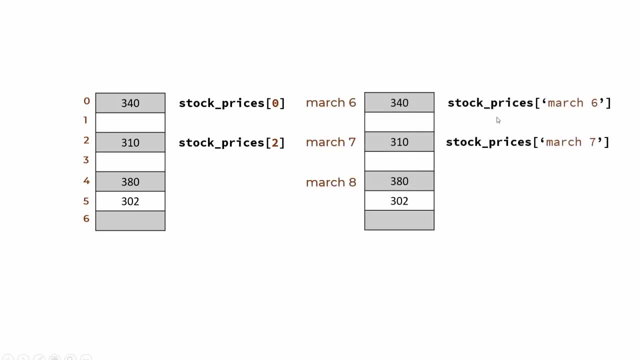 for example, you have a string index and you have a string index and you have a string index. it's ultimately the effect that you're getting is you can use string index in your hash map or hash table. by the way people- sometimes people call it hash map. 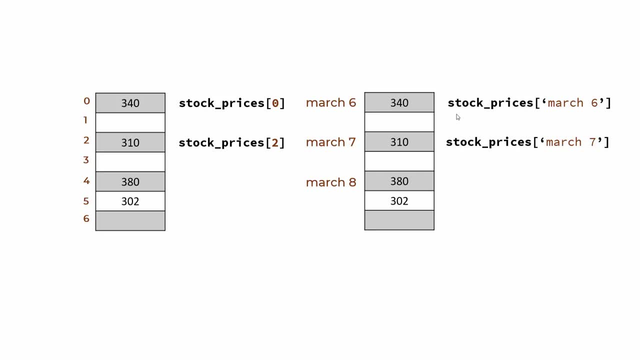 hash table. they all are same. okay. hash table, hash map are internal data structure and dictionary is a Python specific implementation of hash table. so there the question arises is: how did you get number 9 from March 6? so we use hash function. so what is this hash function? there are different ways. 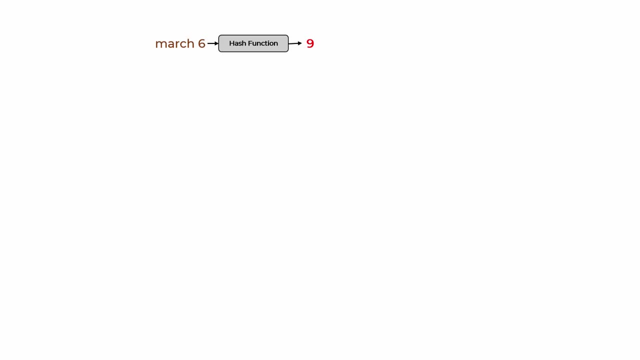 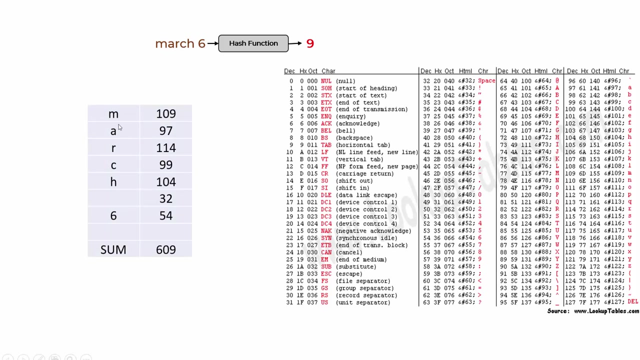 of implementing hash function. I am going to show you one way, which is using ASCII numbers. so I will take each of these letters in this key so you can see March 6, including the space. by the way, for each of this letter, I will find out the. 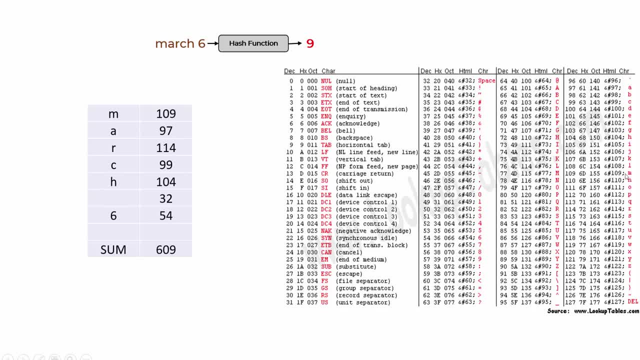 ASCII value. so here in the ASCII table, you can see that the value of M here is 109. similarly a here is 97. I added all this value into a sum and since the size of my array is 10, if you want to get an index between 0 and 9, you all know from 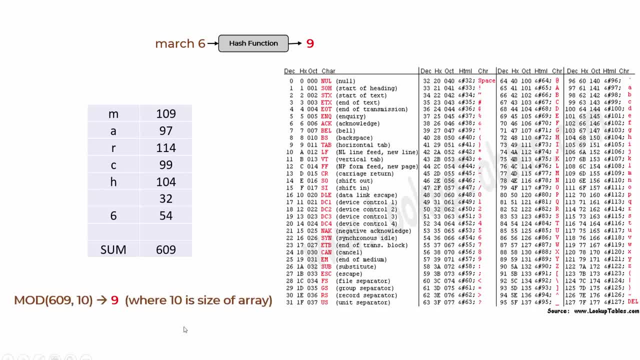 the mathematics that you can do more operation. more operation is nothing, but you are dividing 6 or 9 with 10 and the remainder that you get, which is 9, is your mode. okay, so this is how you generate a 9 from March 6. as I said before, you can use different type of 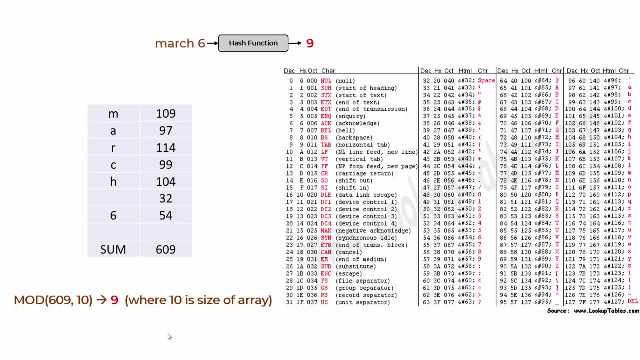 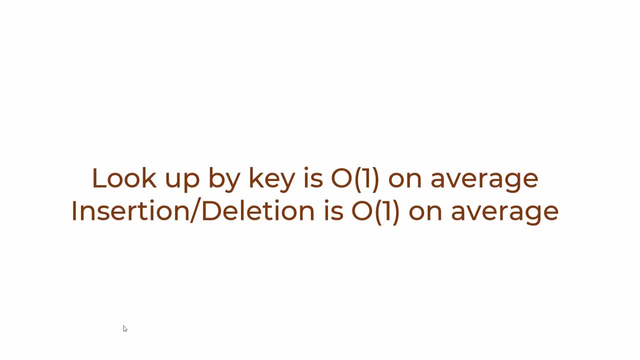 hash function. I just use this particular hash function. okay, so here in the hash map, lookup by key is order of 1 on average. similarly, insertion and deletion is also order of 1 big O complexity on average, and we'll go into this into detail in the next video. so thank you for watching and see you in the next video. 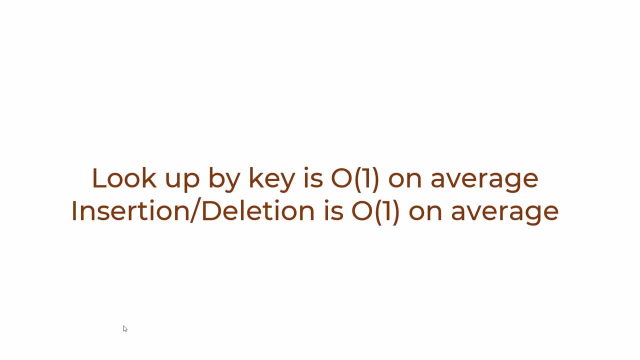 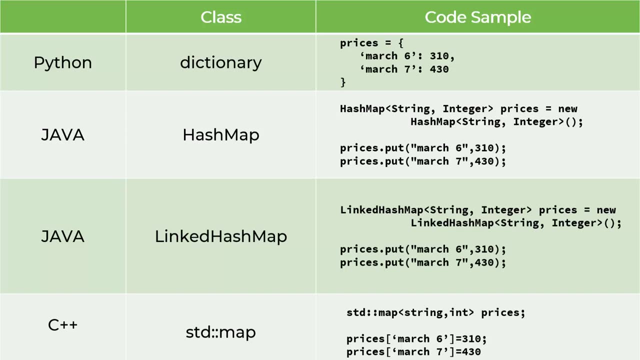 as well. so this is our order. this is an average complexity, but on worst case it might be more than order of 1. here I have list of classes available in different programming languages to implement hash table. in Python, the hash table implementation is called dictionary. here is a code example in: 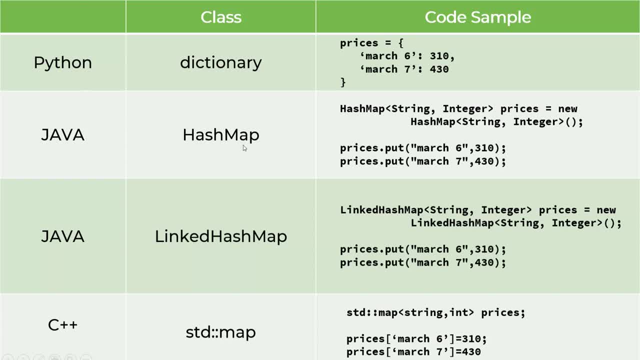 Java you have two classes, hash map and linked hash map, and this is how you create hash mapping in linked hash map. if you want to look at the differences, you can google it. i'm not gonna go in detail on that. in c++ it is called std map. so now let's implement hash map in python. first step of implementing hash table: 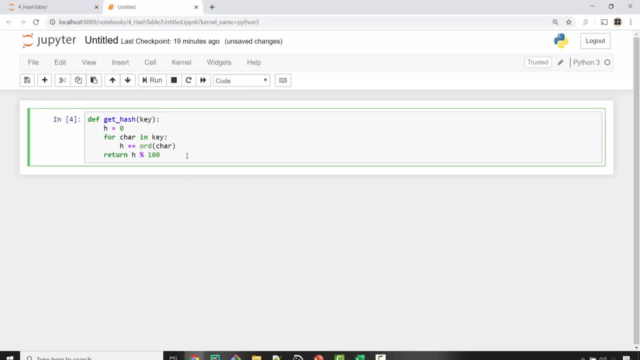 is writing your hash function. so here i have written the same hash function which i showed you in a presentation, which will take a key, which is a string, and it goes through each of the characters and this ord function will just find an ascii value for that character. for example, we 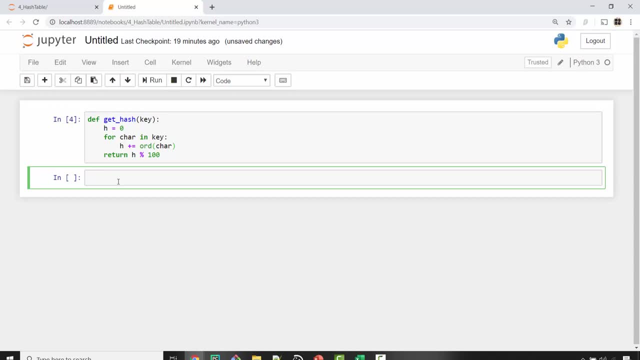 saw that m was 109. so if you do ord of m you get 109 right. similarly, if you do a is 97, so this is giving you the ascii value of a character. so we are going through all these characters in your string doing a sum and that sum we are dividing by. we are doing a mode using 100, so 100 is i am. 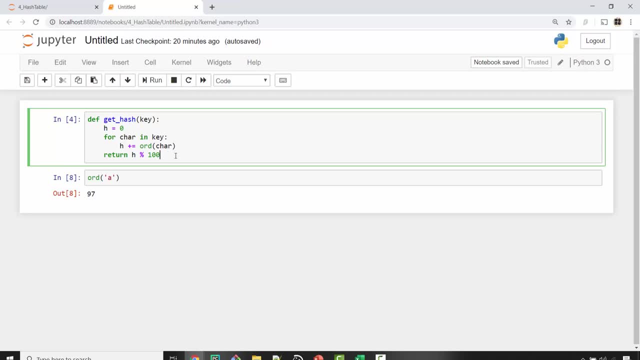 assuming that let's say 100 is the size of my list. right, let's say 100 is the size of my list. right, let's say 100 is the size of my list. right? in the presentation i use 10 as a size, but here we are going to use 100, okay. so what happens is: 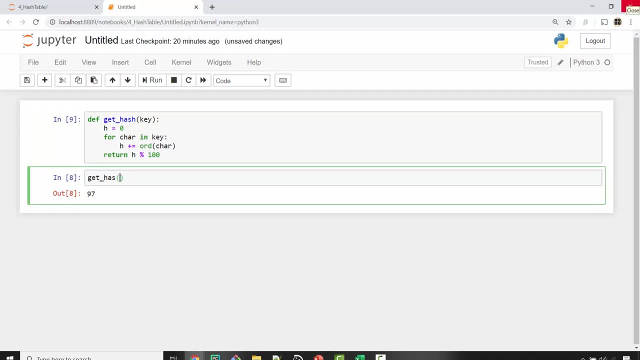 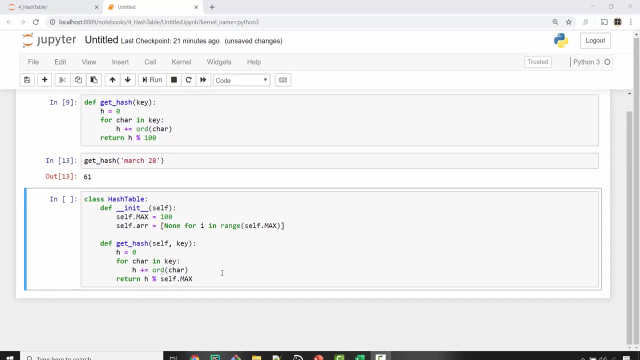 when you call this function, get hash on your key, which is, let's say, match 6. you get this type of value. okay, so you can do different keys and you will get different hash values to implement hash table. i am going to create a class in python now, if you don't know how to create class in python, 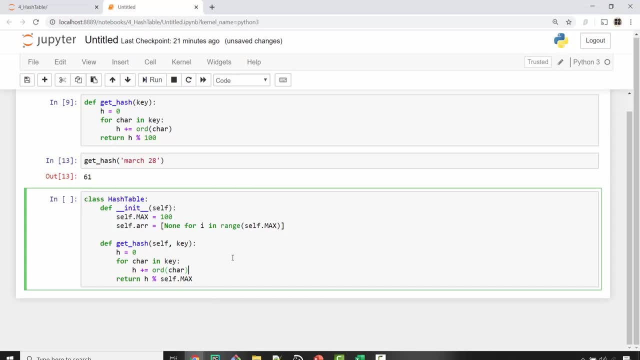 then you can watch my python tutorials. i have tutorials on how to create a class in python, tutorials on classes, list, dictionary and so on, so i'm assuming you have those concepts clear. okay, i created a hash table class where i have this array whose size is 100, and i am initializing 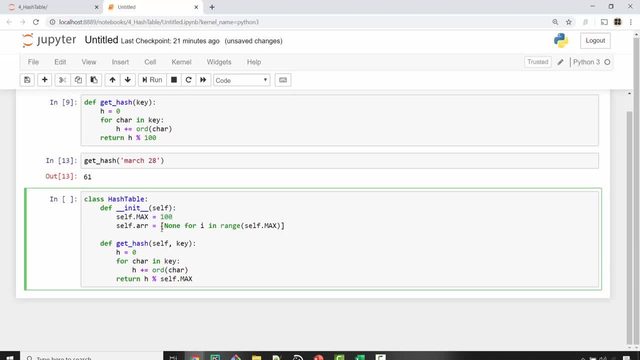 100 elements in this array using list comprehension. here this is how you do list comprehension and the value in each of these elements is none. then i have same hash function which i created here. i i already tested that function, so i'm just copy pasted. i have 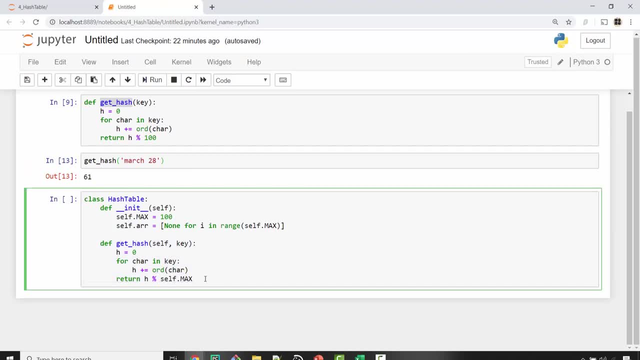 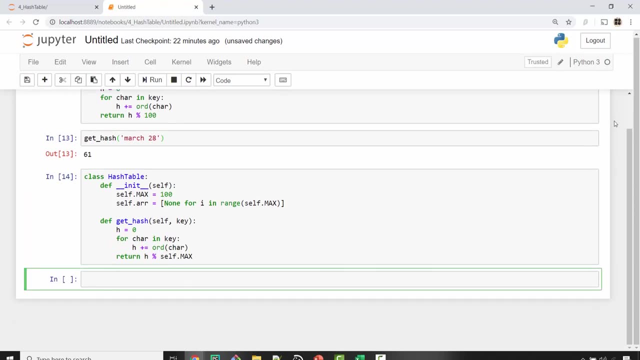 copy pasted that function here. okay, so let's test the this class so far. so i have this class hash map, and the way you can create an object of a class in python is by doing this. now you can do t dot, get hash match six and see you're getting nine. okay, so so far. 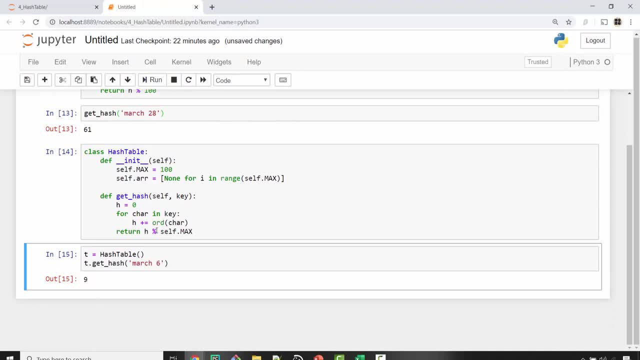 this looks. looks good. now we want to implement a function which can add an item into a hash map and get an item from the hash map. okay, so if you look at our stock prices example, we have day and we have a price. you want to add the day and price. so it is like key value pair. so you want to add a key. 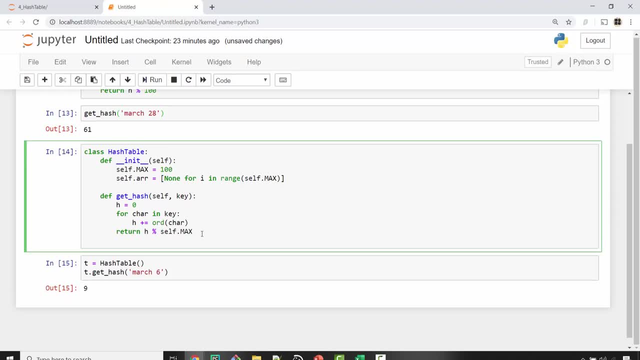 value pair, all right. so for that reason i will define a function called add so key and value. so you want to add a key value pair in your hash map. so first thing you do is you get your hash. so self dot get hash will give you, for a given key, it will give you that hash. so the the way i intend. 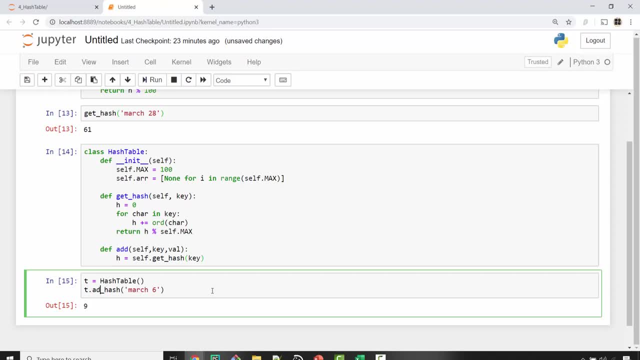 to use. this is i want to say add march 6 some value, and then later on i want to say t dot, get march 6 and it should retrieve me the same value, which will be 130. so that's what i'm trying to do here. so i want to write add and get function. so in add first i retrieved hash, so you know, for march. 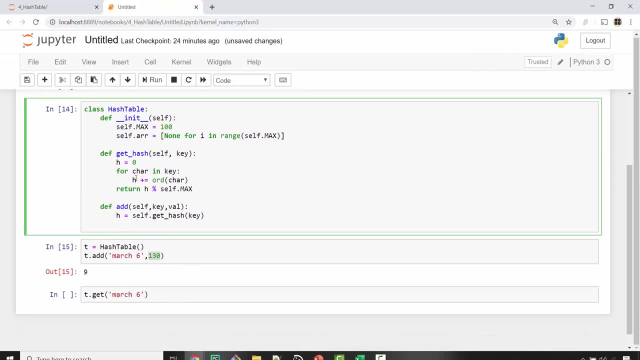 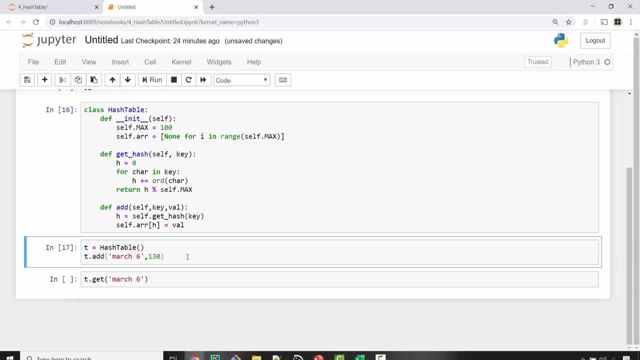 6, the hash will be 9, so i get this 9 index into my array and then all i do is self dot. array h is equal to value. okay, so let's run this by. you can do ctrl enter to run this particular thing and let's execute this. let's. 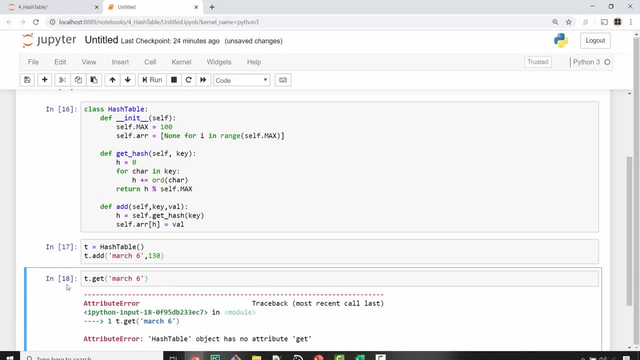 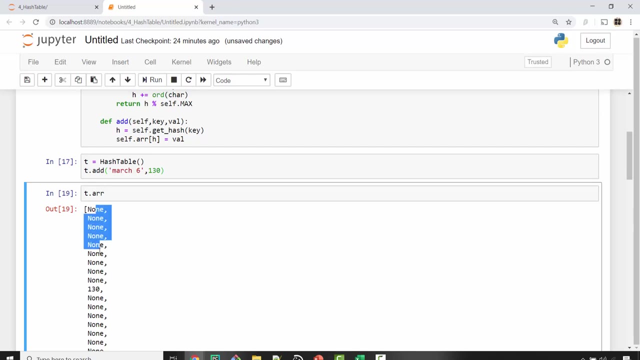 execute this. okay, this function is not defined, okay. so i want to do t dot array and just see what happened to my array. so if you look into it, uh, you see there is 130 value. so at the location number nine. so if you count this, this is ninth location. it inserted value 130 when. 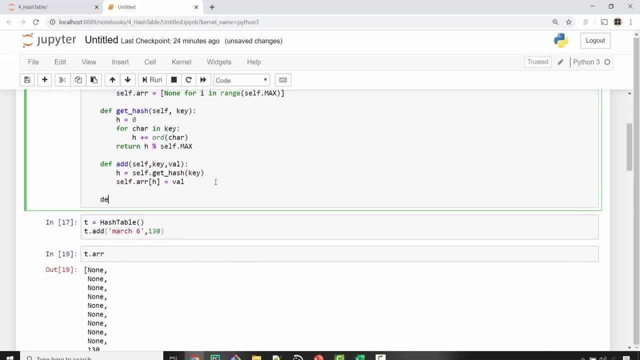 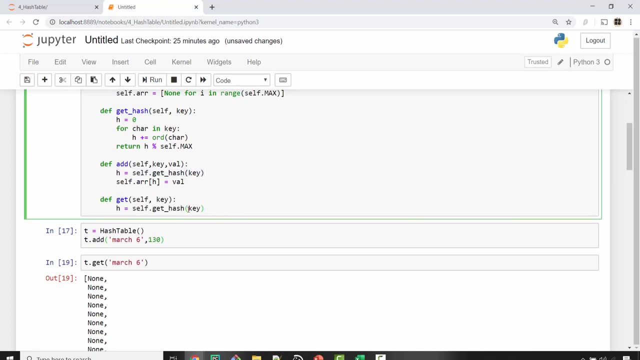 you now call get function. all you are doing is okay. so get function, self and key. because, uh, for get, all you are doing is you are calling it by key and you want to get 130 value. so, as usual, the first step is to get the hash for that key, which is march 6. so this h will be 9. 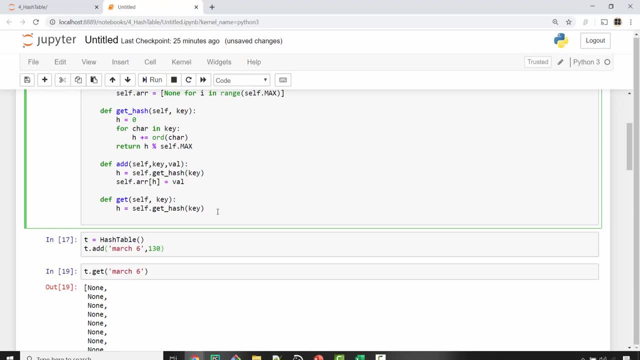 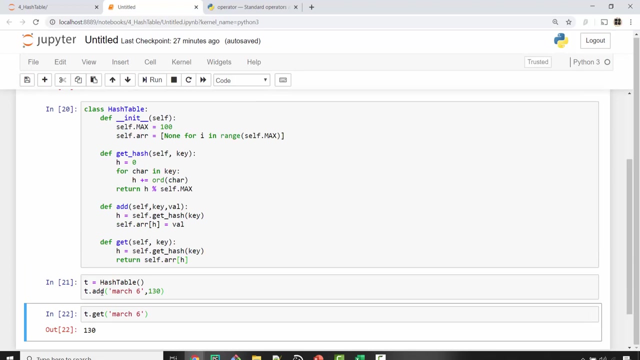 and then you can just return that particular element. so return self dot control enter. this will execute this code again. you have to do control enter here and then control enter here, and now you got your value 130.. so you see, this is this is now working. now, here you are using add and get function, wouldn't it be nice? 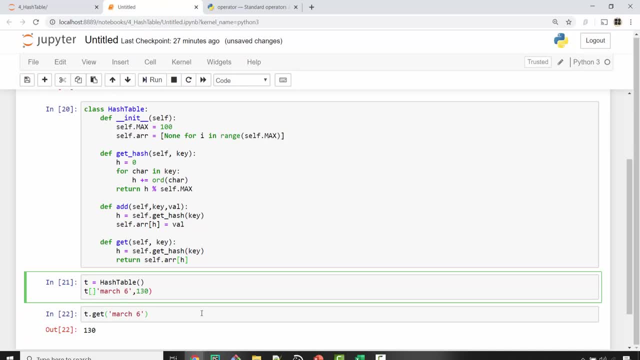 if you can do instead of add, you do something like this. you know how we do it. did that with dictionary. if I have a way of doing something like this, which is something you do usually with your dictionary, that will be little more convenient than calling add and get function. so luckily, Python supports this. 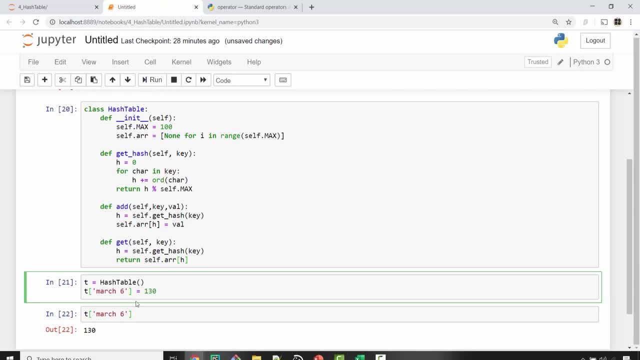 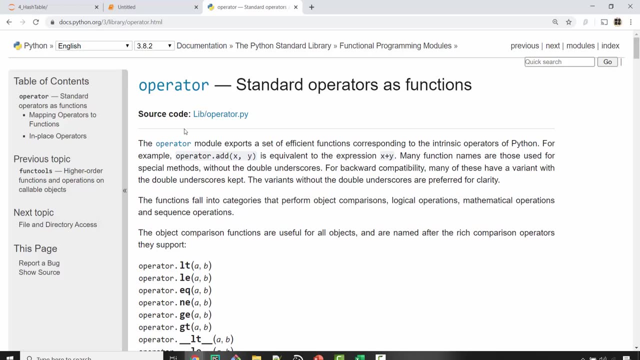 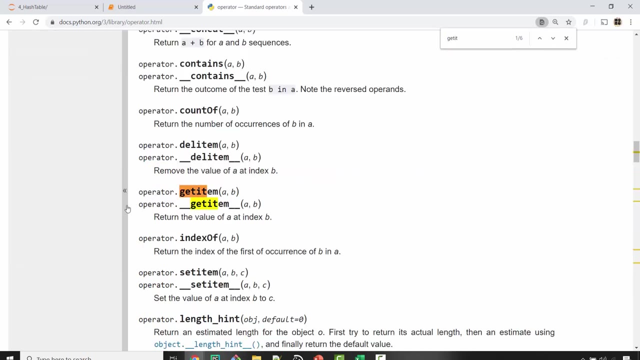 so these are index operators or like item operators which you can override. here I have Python documentation where it shows all the standard operators and here if you look at get item, so this particular function- underscore, underscore, get item- will give you this thing and underscore, underscore, set item. 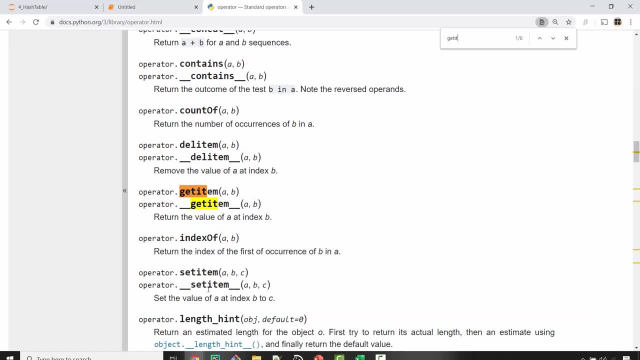 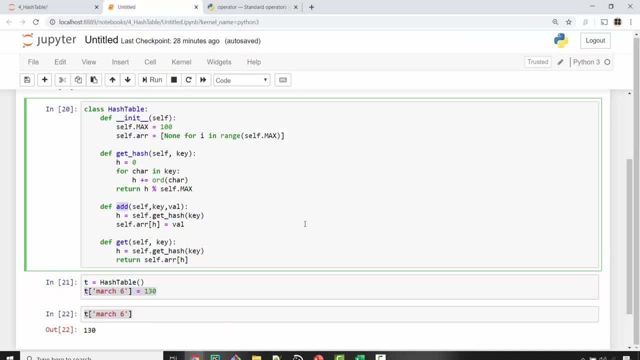 so there is a set item also. this one will will give you this functionality. okay, so all I am doing is replacing add with set item and literally underscore, underscore, get item, get item, underscore, underscore. so control, enter, execute it and now, when I call this, this guy here will call set. 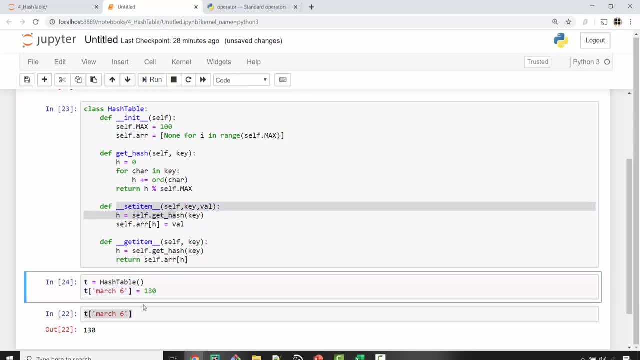 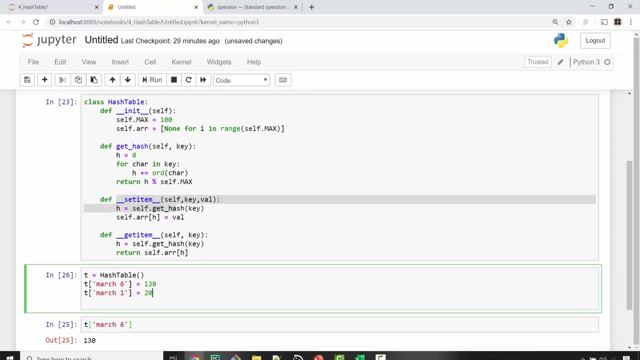 item function. so control enter. so it works and control enter. so see, now this is pretty good. so now let me add a bunch of values. so March 7th, so March 1st is, let's say whatever. okay, I'm just adding a bunch of values here. 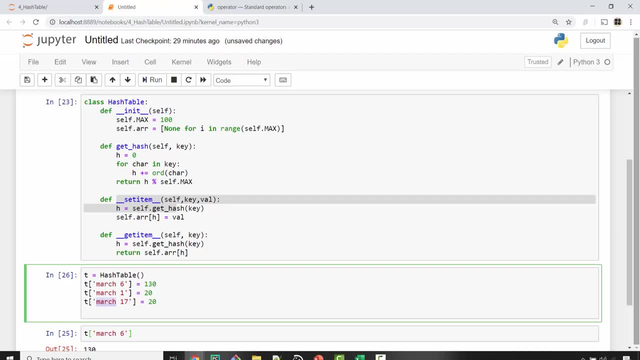 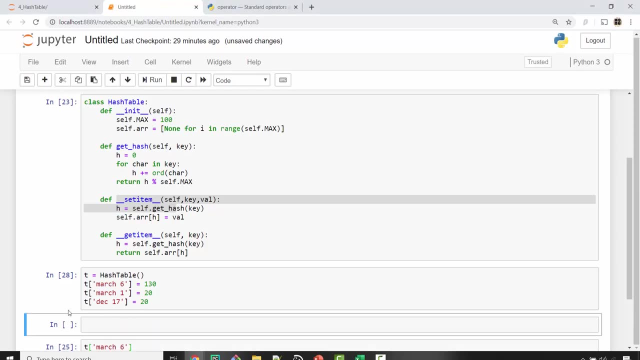 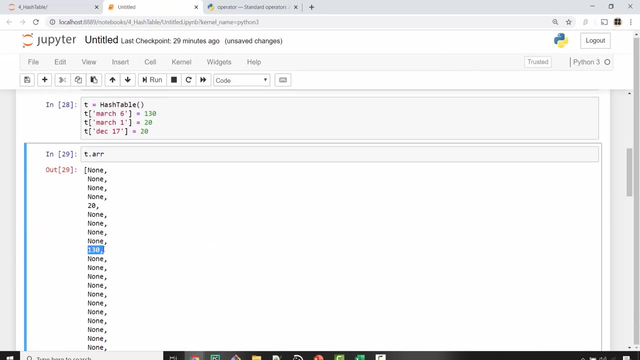 let's say December 17 and so on. and once I do that, I want to look at the status of my array. so t dot array is this: you'll see March 6 got stored at this location. uh, let me just store something else: 27.. so 20, which was March 1, got. 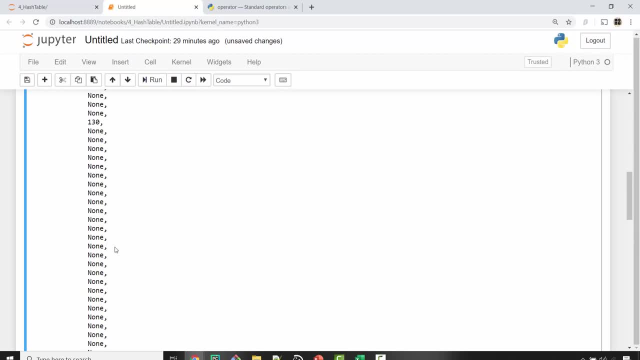 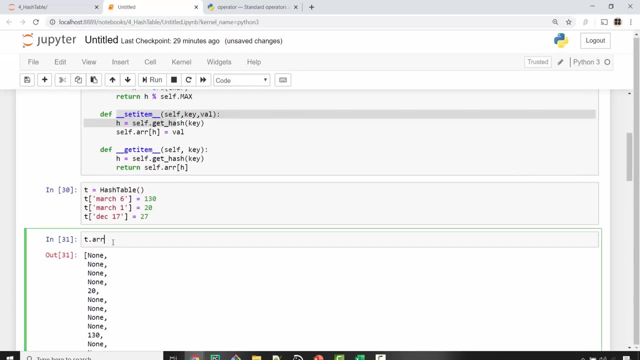 stored here, here see. so hash function gives you these indexes and remaining values are none. but they got stored at different locations here and when you call any of these values you get that back. see: March 1 is this? 17 is okay, so there is no March 17. good, so the it. it returned me none. see, when you do control. 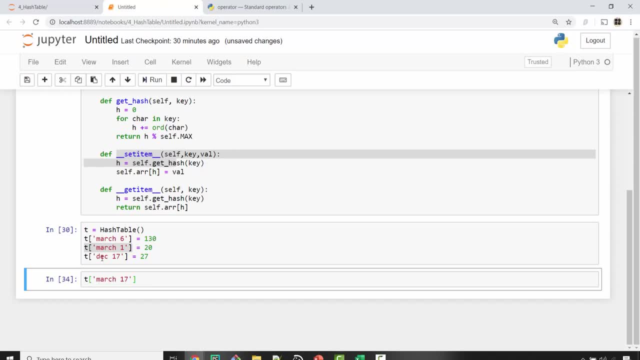 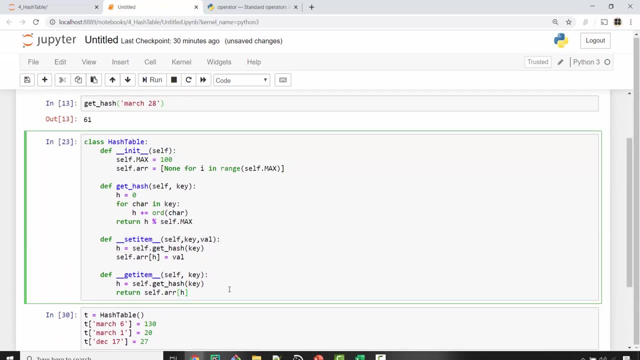 enter, I don't get anything. but if I do December 17, I get 27 back. so by writing this class, what we did is we actually implemented a dictionary. usually when you're doing programming you will be using dictionary. you don't have to define this classes, but by writing this class you get.